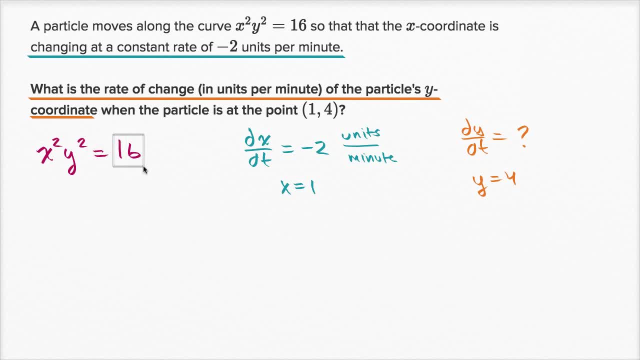 let me just erase this so I have a little bit more. actually, let me just erase this so I have a little bit more, a little bit more space, All right, and so that way I can just add it. So let's take the derivative. with respect to t. 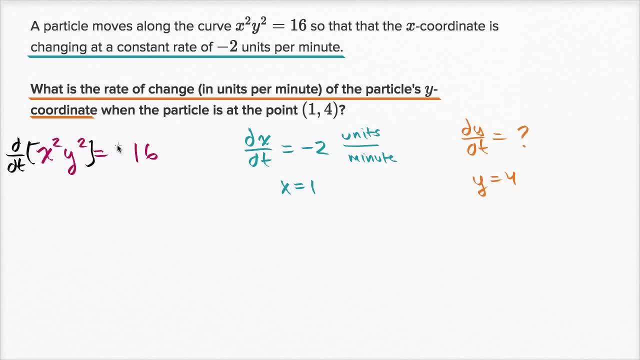 of both sides of that, And if, at any point, you get inspired, I encourage you to pause the video and try to work through it. Well, on the left-hand side, if we view this as a product of two functions right over here we could take the derivative of: 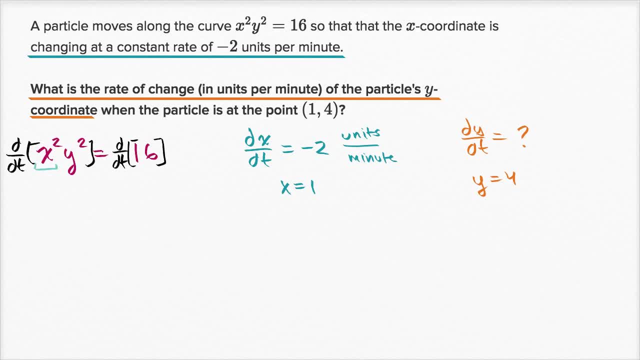 we could take the derivative of the first function, which is going to be the derivative of x squared with respect to x, so that is two x. And remember, we're not just taking the derivative with respect to x, we're taking the derivative. 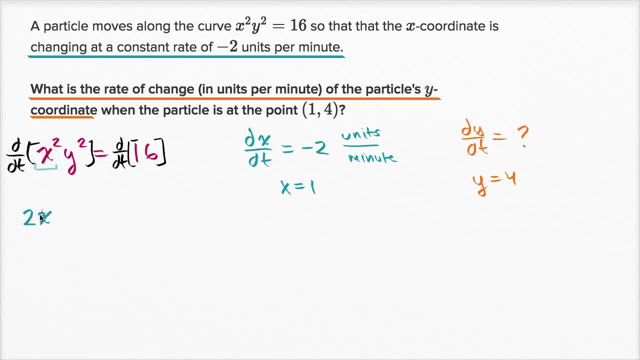 with respect to t. So we're gonna have to apply the chain rule. So it's gonna be the derivative of x squared with respect to x, which is two x times the derivative of x with respect to t. So times dx, dt. 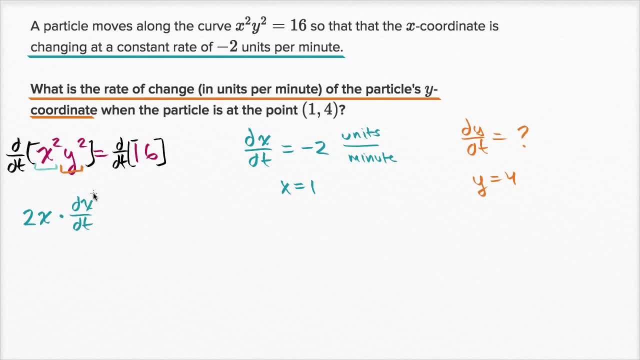 And then we're gonna multiply that times dx, dt. That's the second function, So times y squared, times y squared, And then that's gonna be plus the first function, which is just x squared times, the derivative of the second function with respect to t. 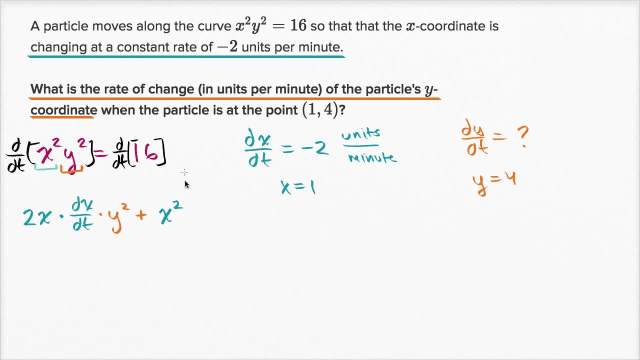 And so, once again, we're gonna apply the chain rule. The derivative of y squared with respect to y is two y. Let me do that in that orange color. It is equal to two y, And then times the derivative of y with respect to t. 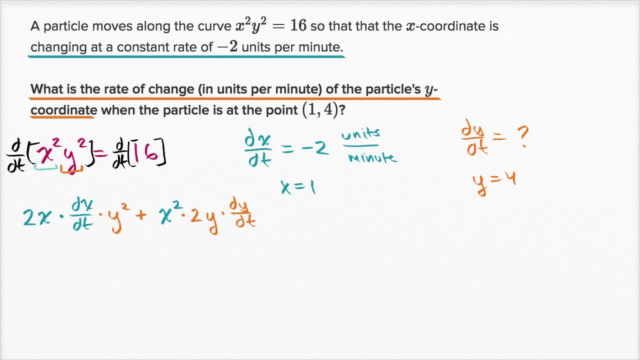 Times dy dt. And then that is going to be equal to, that is going to be equal to the derivative with respect to t of 16.. Well, that doesn't change over time, So that's just going to be equal to zero. 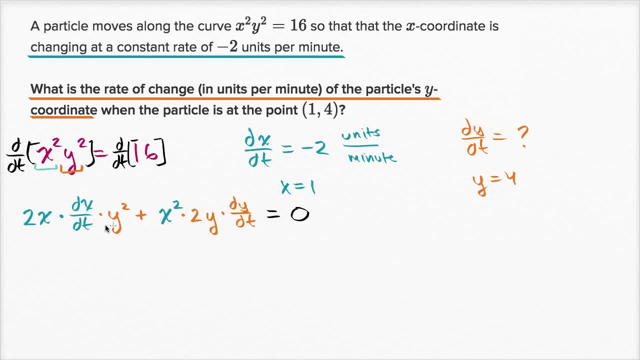 And so here we have it. We need to simplify this a little bit, but we have an equation that gives a relationship between x, derivative of x with respect to t, y and derivative of y with respect to t. So actually, let me just rewrite it one more time.